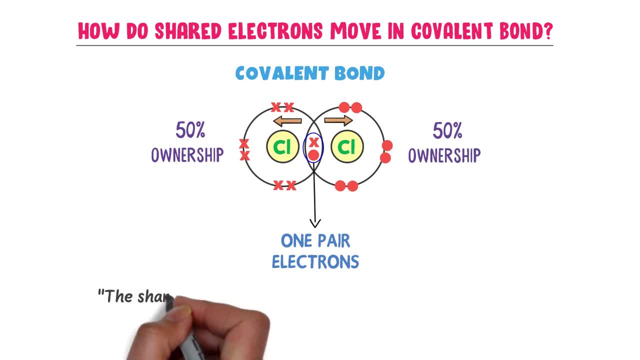 shared electrons. Therefore, we say that the shared electrons move in the orbitals around both the atoms. Let me repeat it: the shared electrons move in the orbitals around both the atoms. For example, these shared electrons would revolve around this chlorine atom and. 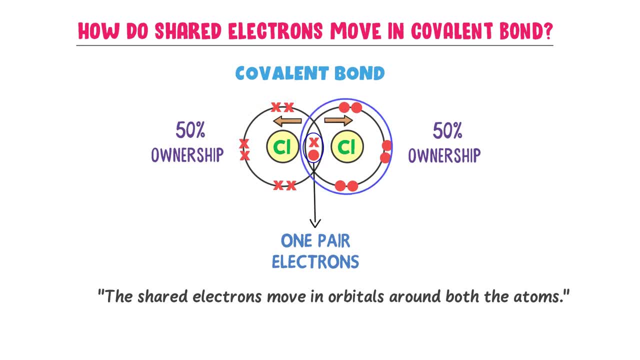 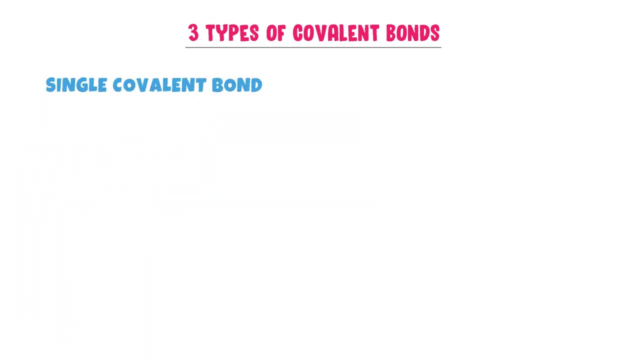 also, these shared electrons would revolve around this chlorine atom. So therefore we say that these shared electrons belong to both the chlorine atoms. Now let me teach you the three types of covalent bonds. The first type is single covalent bond. 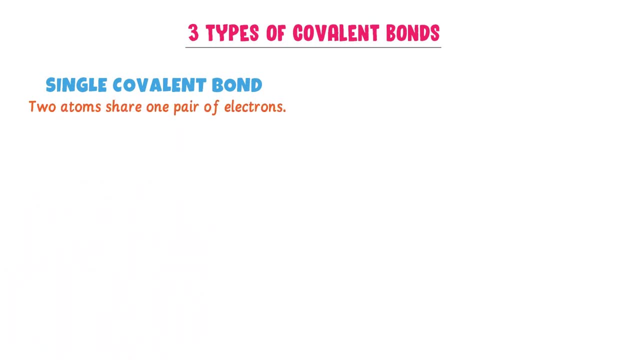 It is the covalent bond in which two atoms mutually share one pair of electrons. For example, consider two hydrogen atoms. We know that this hydrogen atom has one electron and its last shell, and this hydrogen atom has also one electron and its last shell. Now, 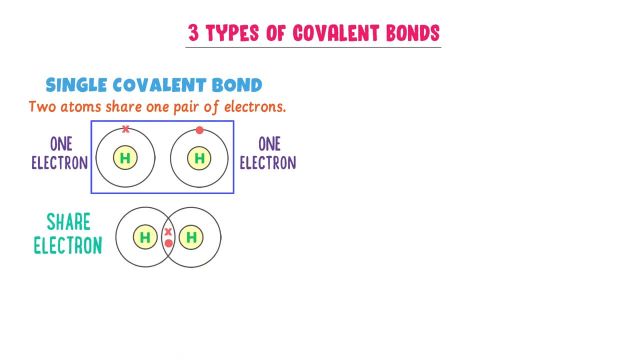 they would combine together by mutually sharing one electron each hydrogen atom to form a covalent bond. So we can see that this is the one pair of electron shared between two atoms of hydrogen. Here the duplicate rule of each hydrogen atom is completed. So they have. 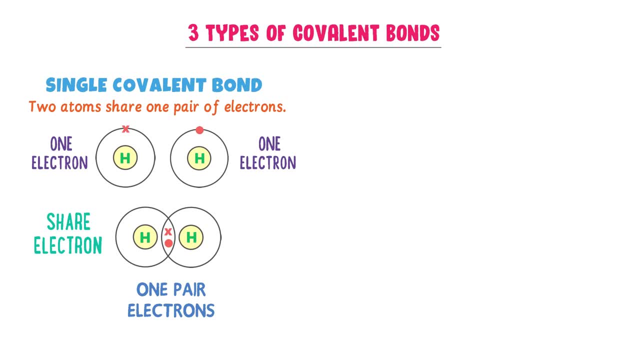 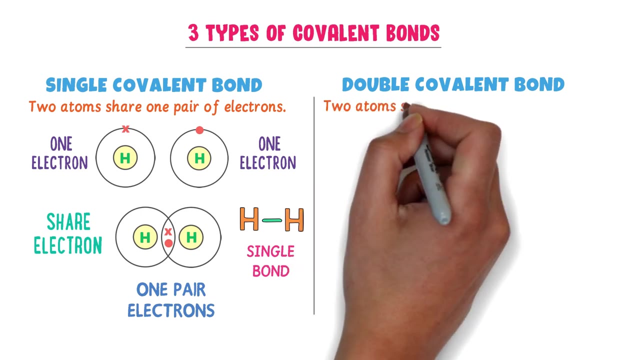 formed a hydrogen molecule. Remember that this hydrogen atom has one electron and its last shell. Remember that a single straight line between two hydrogen atoms shows single covalent bond. Now the second type of covalent bond is double covalent bond. It is the covalent bond in which two atoms mutually share two pairs of. 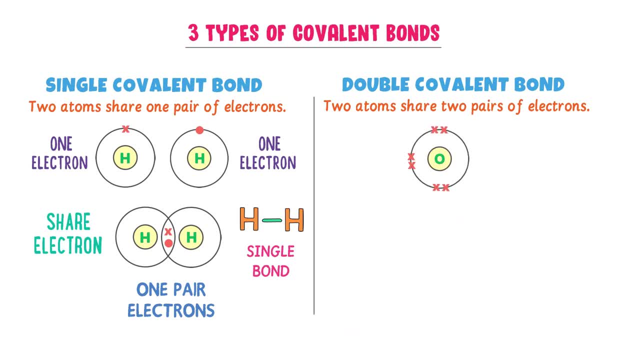 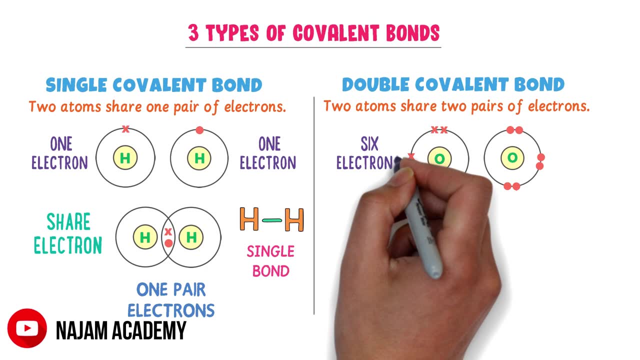 electrons. For example, consider two atoms of oxygen. We can see that in the last shell of this oxygen atom there are six electrons present. It needs two more electrons to get stability. Also, in this atom of oxygen there are six electrons present. It also needs two more electrons to get stability. Now they would. 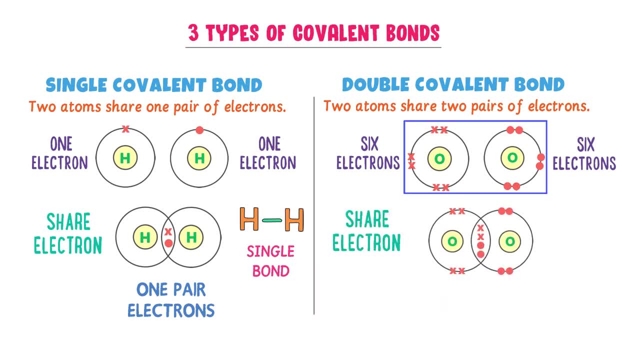 combine together by sharing two electrons each oxygen atom to form a covalent bond. So we would get this molecule of oxygen gas. Here we can see that this is one pair of shared electrons And this is another pair of shared electrons, So there are two pairs of shared electrons.